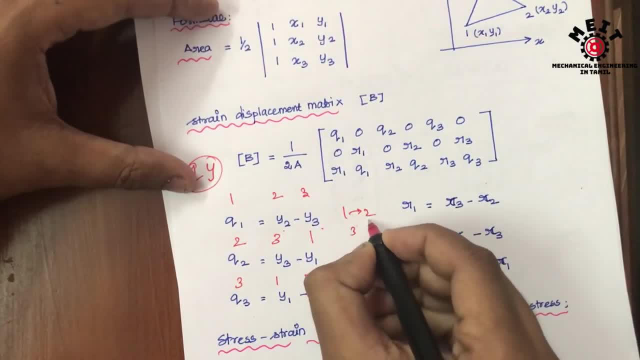 So it is a circle like 1,, 2, 3.. After 2 it is 3,, after 3 it is 1.. So after 1, there will be 2, there will be 3.. After 3, there will be 1, 2.. 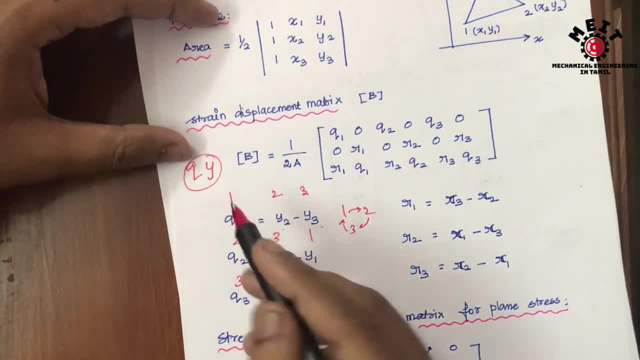 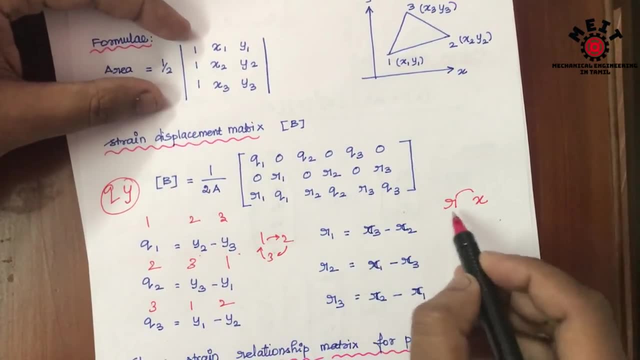 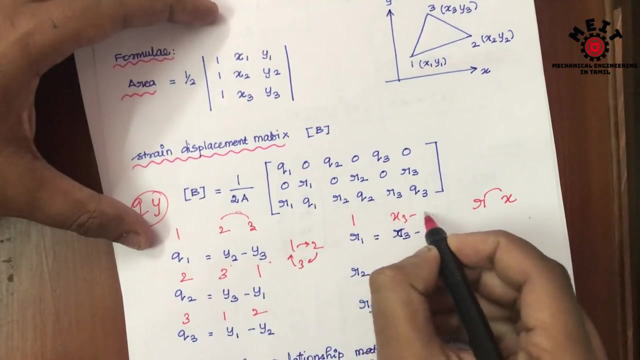 Q1, y. that will be related in shapes and similarly, if we look at R, its shape will look like X, so R will have X. similarly, if we put 1,, 2,, 3, we will put it as inverse, like X3-X2. 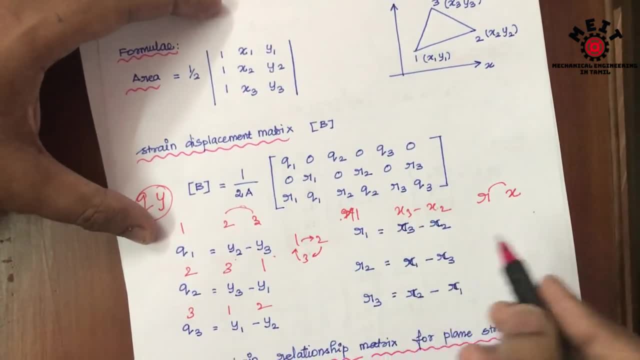 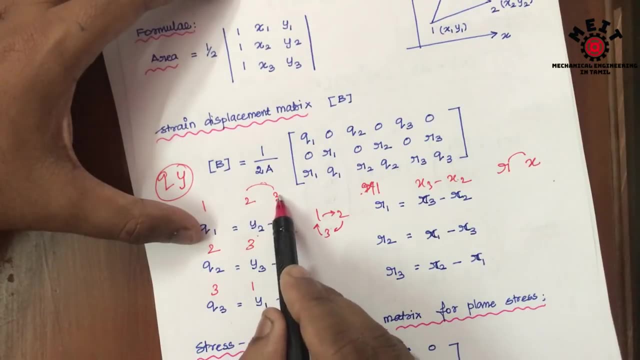 that is R1, so R1 will be X3-X2. in the previous case, 1, 2, 3, 2, 3, 1, 3,, 1, 2 will be a cycle. in this cycle, if we put 1,, it will be 2, 3, but 3, 2 will come. 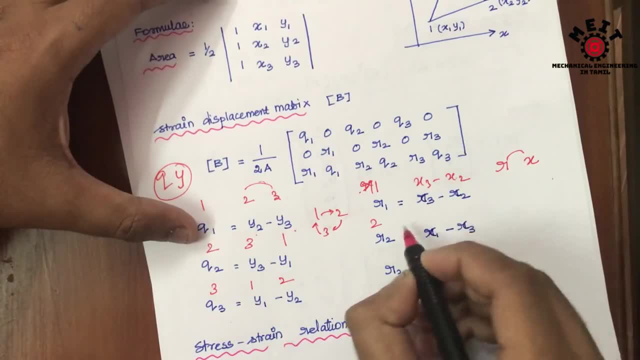 then if we put 2,, it will be 3, 1, so the inverse will be 1, 3. then if we put 3, it will be 1, 2. the inverse will be 2, 1- X2-X1. 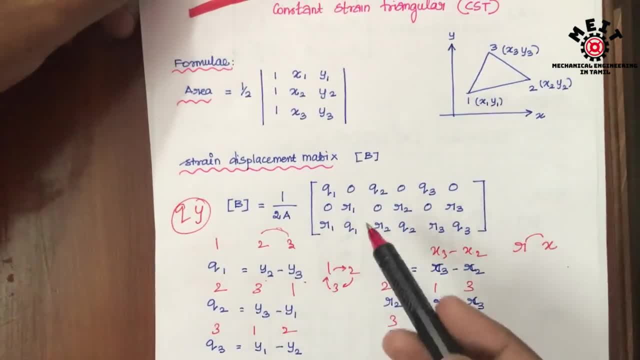 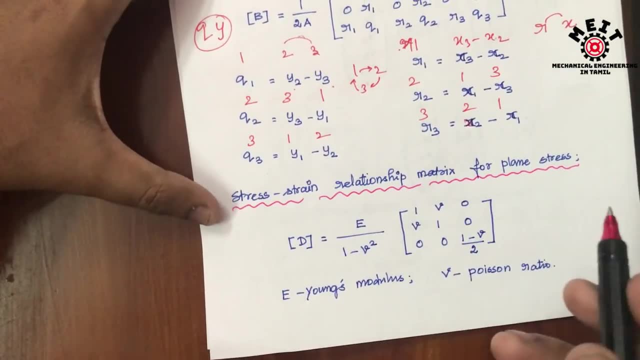 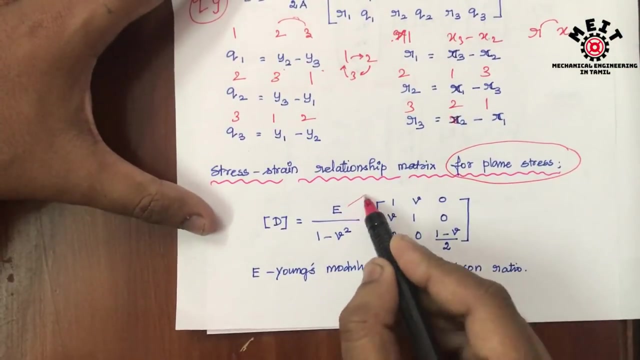 so that is the way we can remember the formula for Q and R which is in the strain displacement matrix. so this is the formula for beam matrix. then stress, strain relationship formula for plane stress condition. some people mention about plane stress or plane strain. so in the formula E is the Young's smallest value. 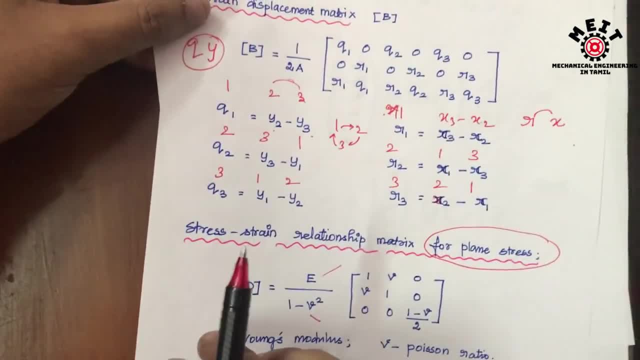 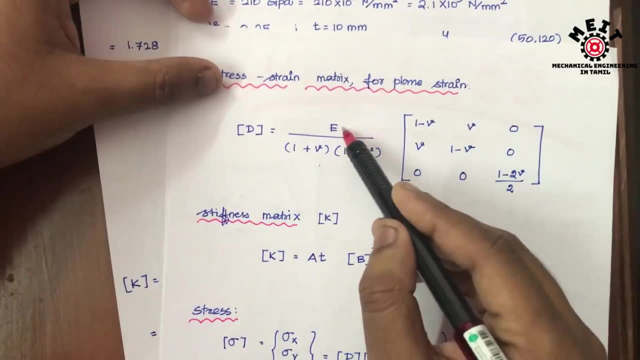 Mu is the Poisson ratio and this is the matrix for stress strain relationship. and this is the matrix for stress strain relationship. and then if we take plane strain, there is a difference from the formula. so E is the Young's smallest and Mu is the Poisson ratio. 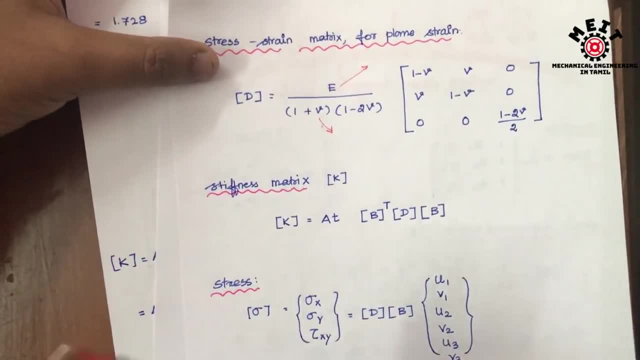 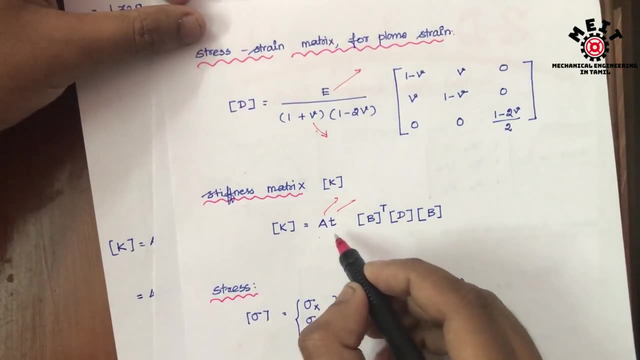 we have to substitute the value and we can get the beam matrix. so to find the stiffness matrix the formula will be like: K is equal to A into T. E is the area, T is the thickness of the plate, particular element. so area into thickness of the element, into. 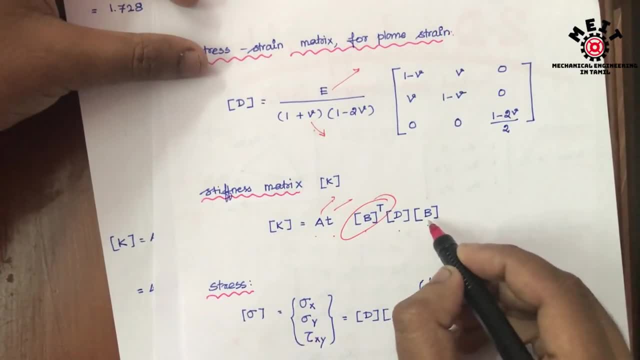 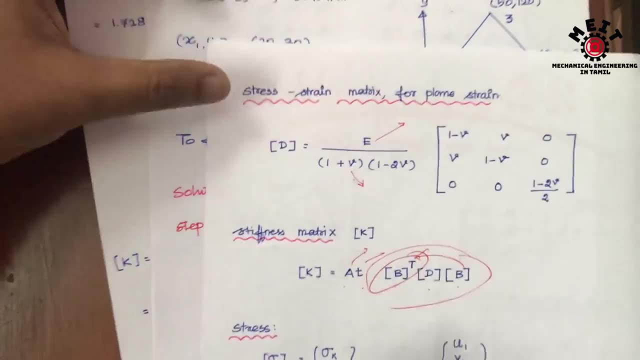 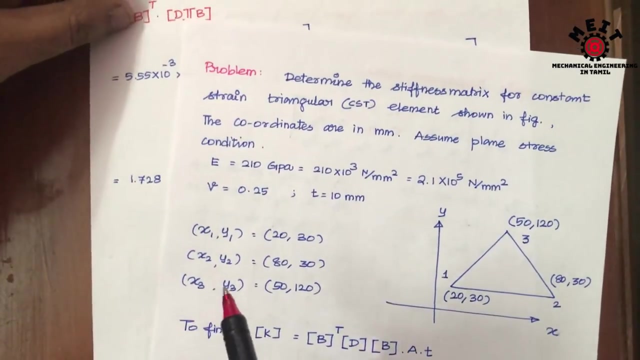 transpose of beam matrix, then D matrix, then B matrix. B matrix will be transpose. we have to multiply all the 3 matrix and we can get the K matrix. so now let us take an example of how to find the K matrix. so here, determine the stiffness matrix for constant strain. triangle element. 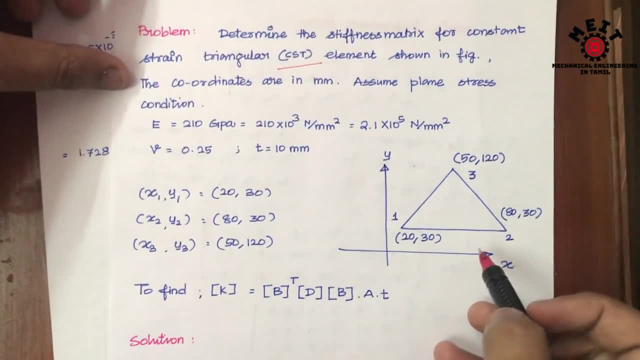 that is CST element, as shown here. in this formula there are 3 points: 1, 2, 1, 3. 1 will be 20, 30. 2 will be 80, 30. it is a horizontal line, so 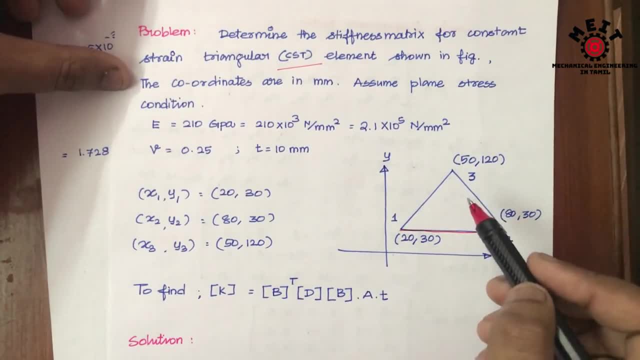 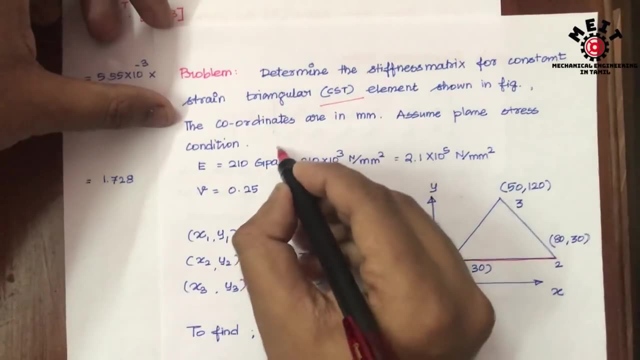 and then 3 will be 50, 120. they have mentioned 3 corners. that is the CST element. so the Young's smallest value 220, 210 jihapascal, that is 210 into 10 power, 3. mehapascal, that is 210 into 10 power, 3 Newton per ohm square. 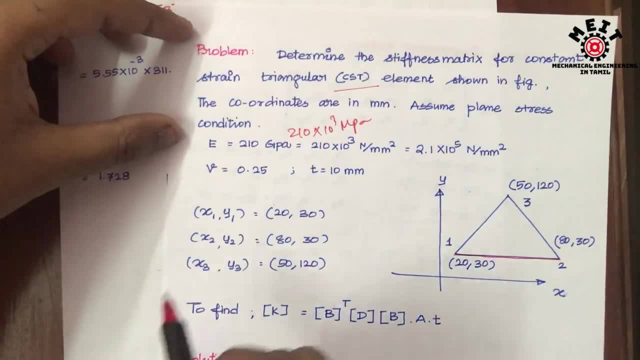 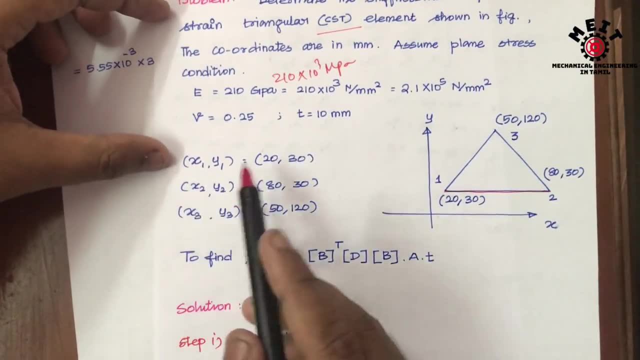 so 2.1 into 10, power, 5 Newton per ohm square and Poisson ratio is given 0.25. then thickness value of the plate is given 10 mm and all the coordinates I can consider 1 as 1, 2 as 2. 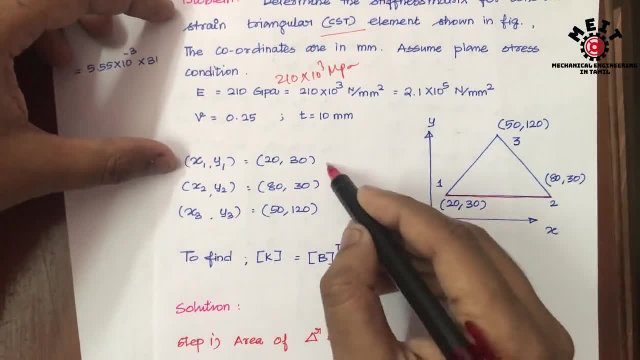 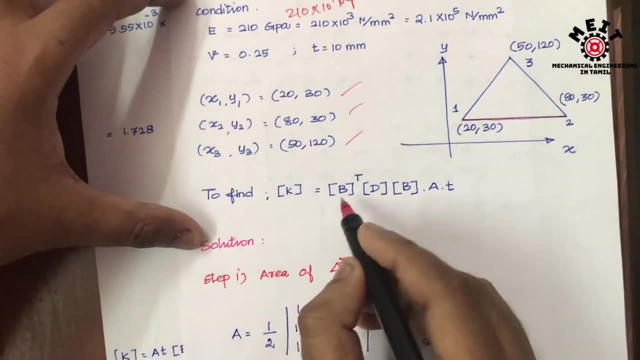 X1, Y1, there is a point- and X2, Y2, X3, Y3, so that is the coordinates. so what I have to find is I have to find the stiffness matrix. stiffness matrix formula is transpose of B matrix, D matrix and B matrix. 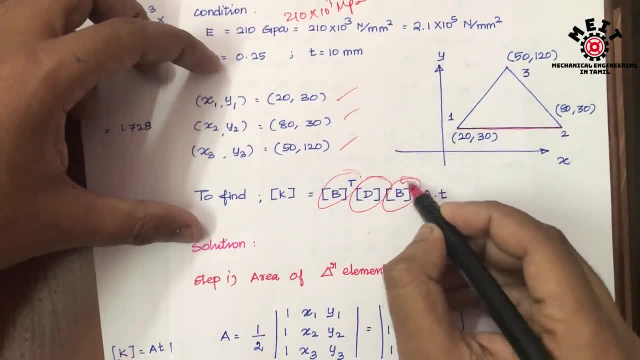 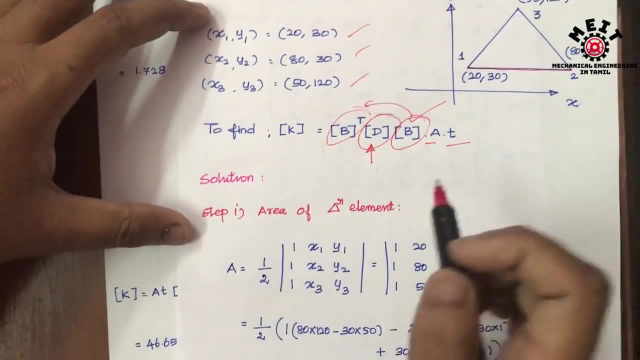 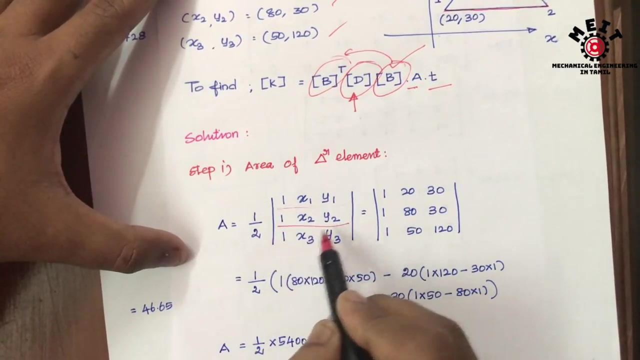 into area, into thickness. so I have to calculate B matrix, then transpose of that one and then D matrix. so let me find that first area first. so area is like area, formula 1 by 2 into determinant of 1X1, Y1, 1X2, Y2, 1X3, Y3. 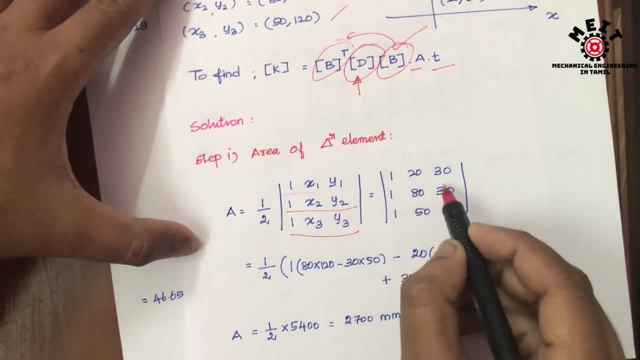 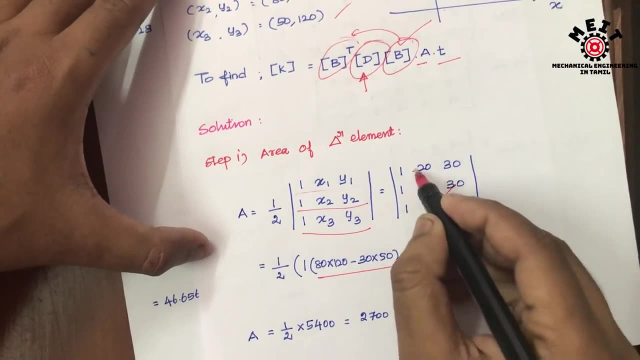 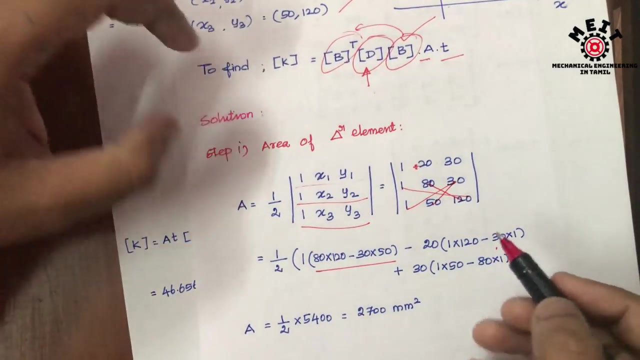 so I can put the formula and determinant value like 1, 1 into 80, into 120, minus 30 into 50 and similarly minus 20 into minus 20, into 1, into 120, minus 30 into 1. so you know how to calculate determinant of the matrix. 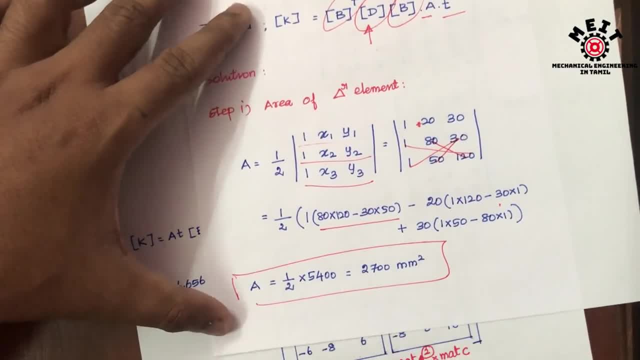 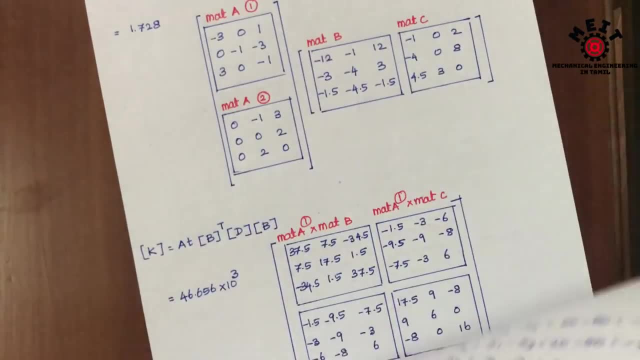 so there is a formula for A and you can calculate the value that A is 2700 mm square. and after calculating A I need to calculate B matrix, then D matrix, so B matrix find I can write the formula simply 1 by 2A, like Q0. 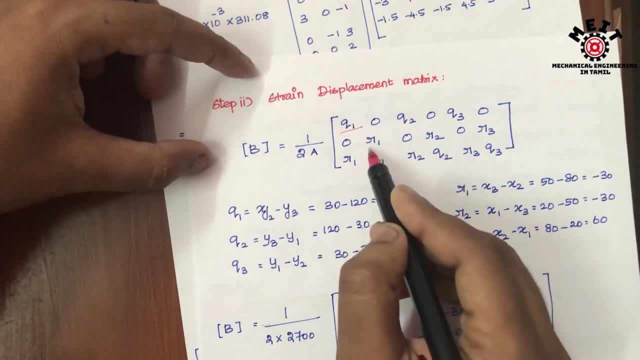 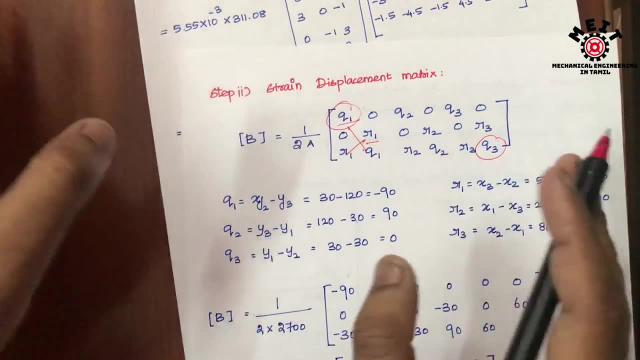 Q2: 0 and Q3: 0- 0 R1. so first start in Q and then 0 R1. then R1 comes here, Q comes here. so Q will be in starting and Q will be in ending. keep this in mind. so that is the way of formula. 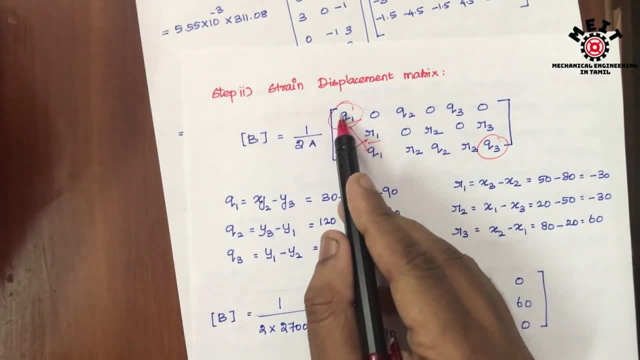 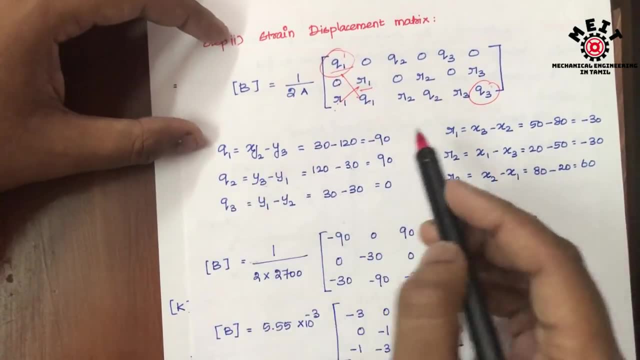 don't forget to write Q here and R here. it always starts from Q and end with Q. that's it. and then already I said that how to memorize Q and value Q to value, I have to remember this formula like 1, 2, 3. 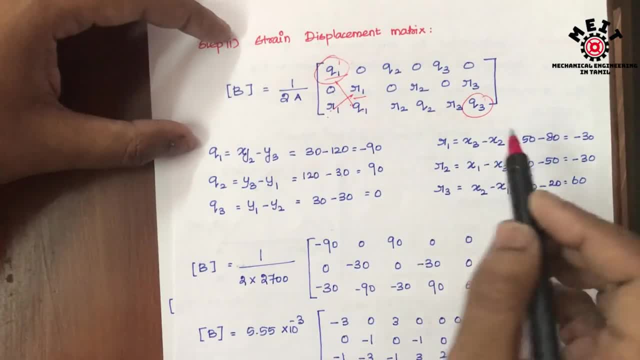 2, 3, 1, 3, 1, 2 or 1, 2, 3, 3, 2, 2, 3, 1, like that, like that, everyone. I have explained that you memorize the formula and get the value for Q1 to Q3. 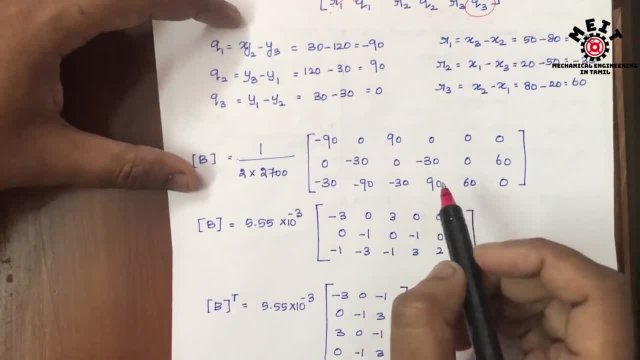 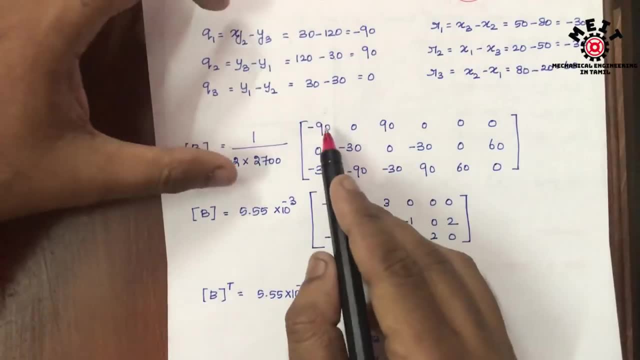 I mean R1 to R3. you find the value, you substitute the value and you can take the common out like 90, 30, 90, 30, 30 will be the common one, so I can take the 30 out. so if I take out 30, 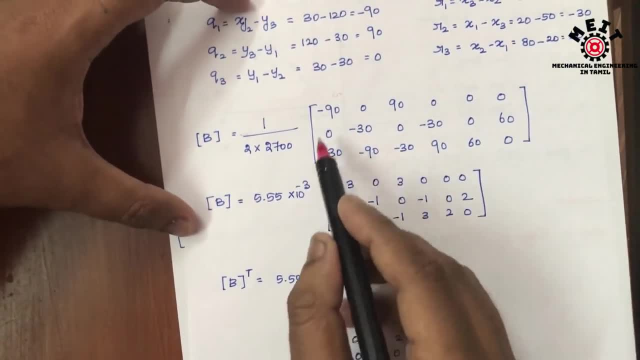 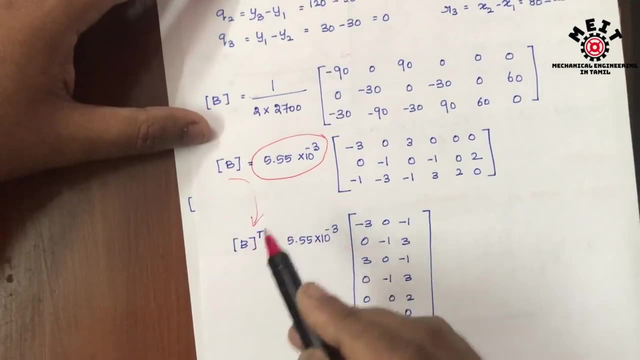 there will be only 3, so minus 3, like 0, 3. and if I take out 30 and simplify everything 5.55 into 10 power minus 3, then there is a matrix. so transverse matrix will be Bt and if it is column. 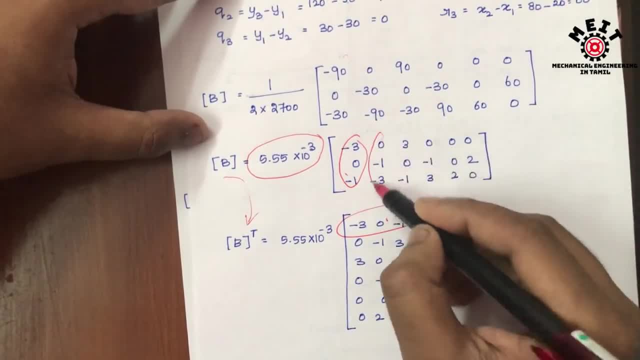 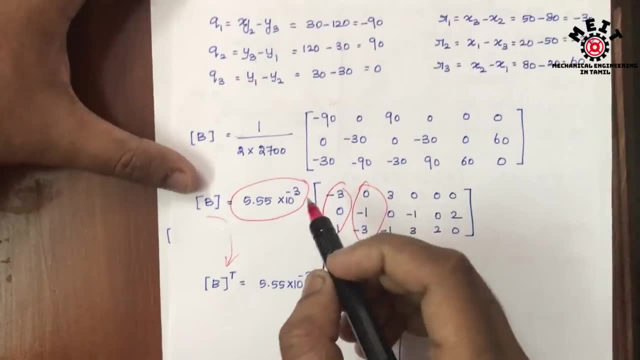 it will be row that is, first column will be first row and second column will be second row and like that we have to like return. that's it, that is Bt. so B matrix- find one term. Bt matrix: find one term. so I need to find. 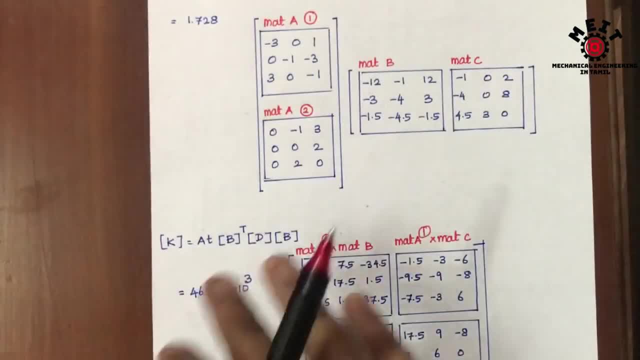 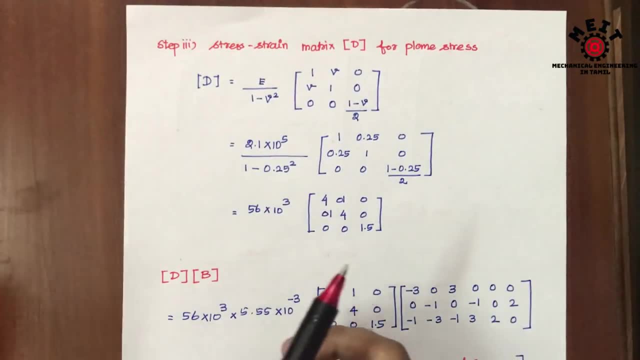 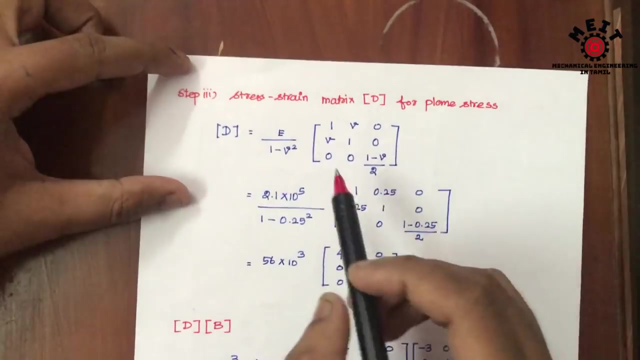 D matrix. then I have to do the multiplication. that is step number 3. step number 1 will be area and step number 2 will be like B matrix and Bt matrix, and step number 3 will be stress strain matrix. that is D matrix. so I have put that. 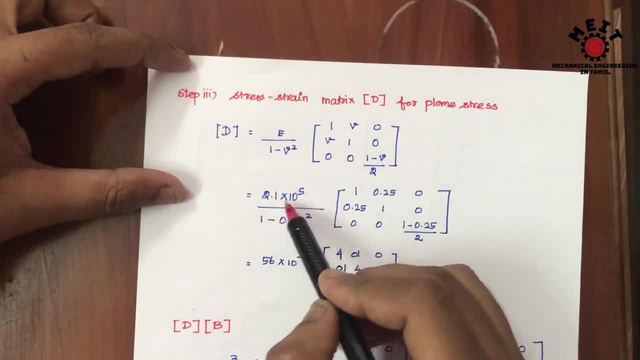 I have put the formula E and 1 minus mu- square E value is the smallest value, 2.1- into 10 power 5 and mu is the Poisson Ratio. it is given in sum 0.25 when I put all the value in the matrix formula. 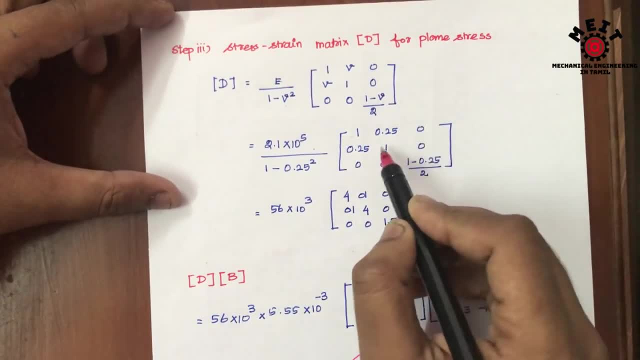 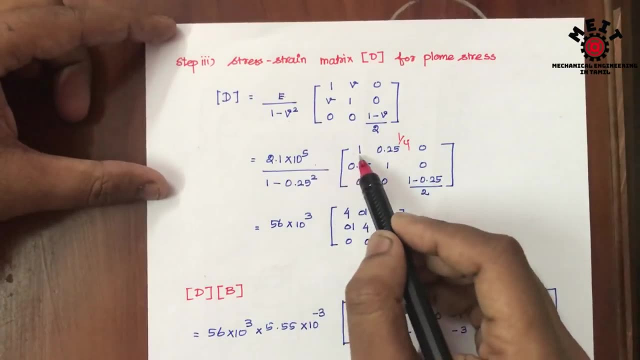 I can get it like 1.25 or 0.25 is 1 by 4, like that. so what I will do is, if I take 0.25, as common that will be, if I take 0.25 from 1, it will be 4 times. 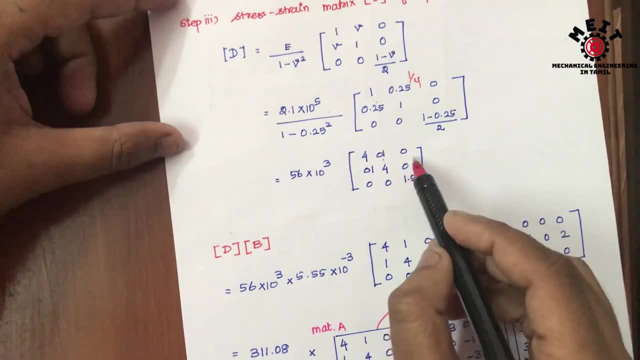 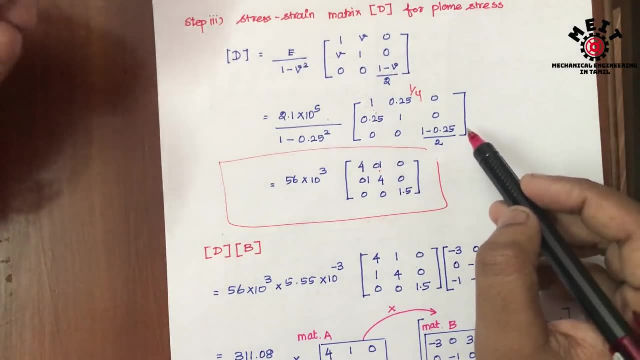 so 4. if I take 0.25, it will be 1. so if I take 0.25 out, I can simplify the matrix like that: you can take out any value that is convenient for you. if not, if you can't take it out, 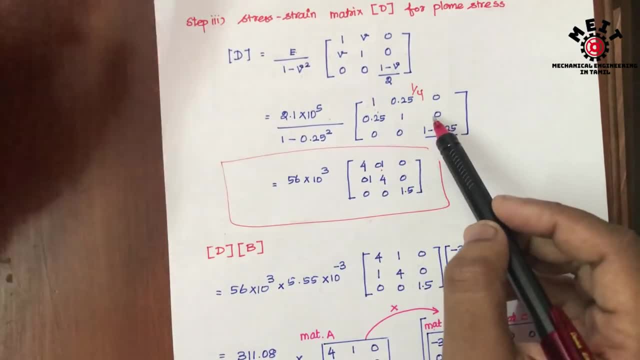 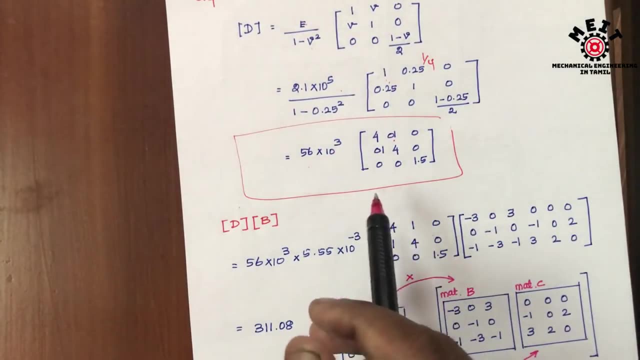 you can keep that value inside. so 10 power, that will always be out of the matrix. that will be more convenient for us. so to simplify everything, 56 and 10 power 3, then 410, 140, 0015, the matrix comes. then what is my? 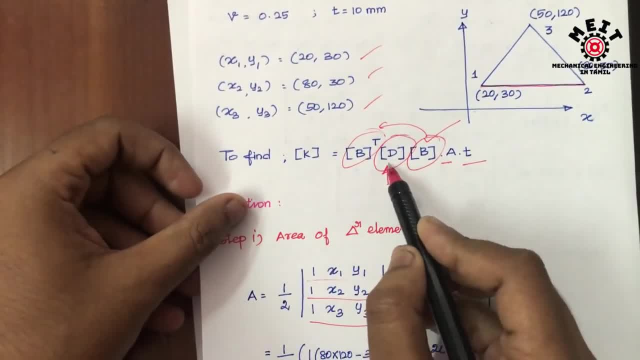 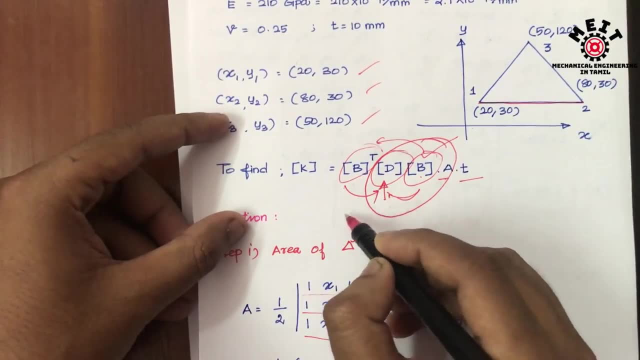 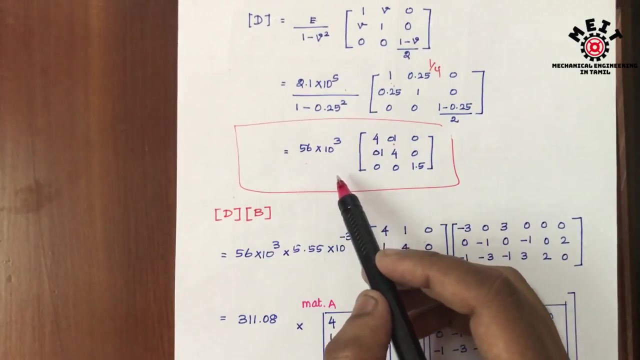 stiffness matrix K is equal to Bt, Db. so first I will find what is Db after completing Db matrix with Bt. if I multiply that answer I will get the total matrix. so let me consider Db first. so D value 56 into 10 power 3. 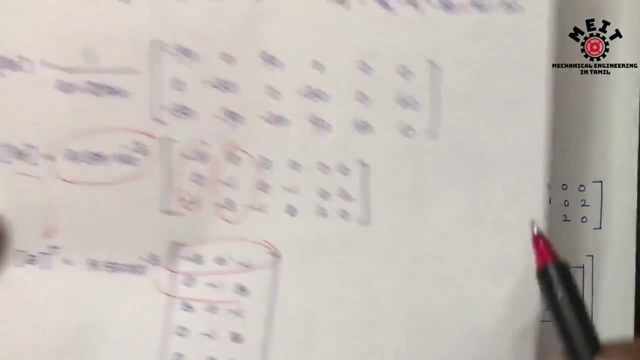 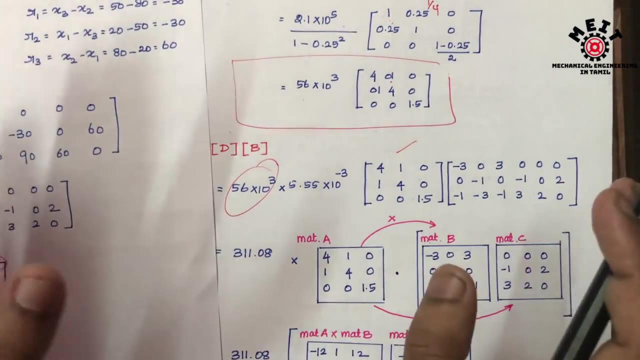 if I put that value then the matrix is there. and similarly B matrix is 5.55 into 10 power minus 3, then the matrix so 5.55 into 10 power minus 3 in that particular matrix, then I have put that. so how to. 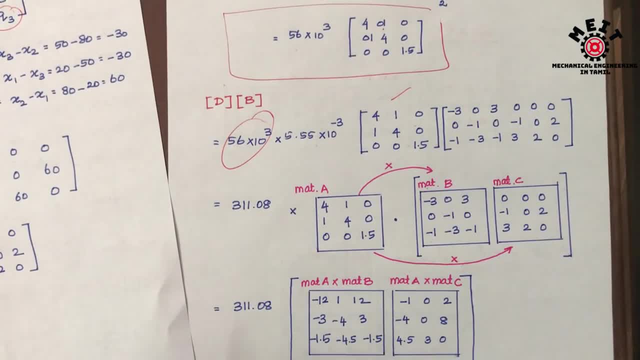 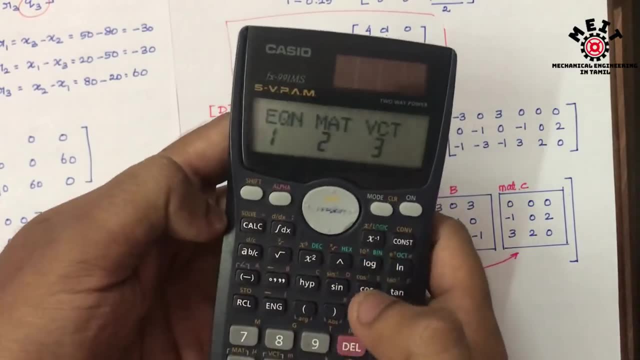 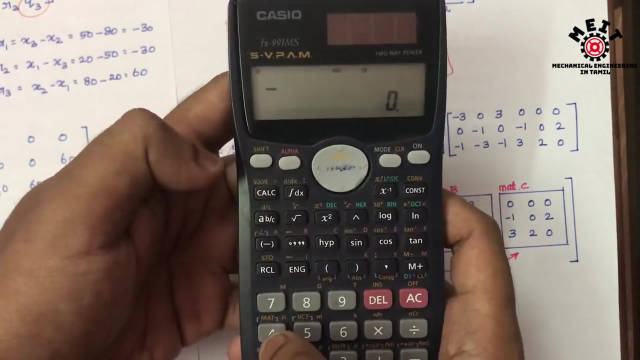 multiply this. how to use this in calc, I will tell you so we can go with like that, in more like 991 ms. in this calc there will be matrix, so be careful on that. so then more go for matrix and then shift 4 so we can define. 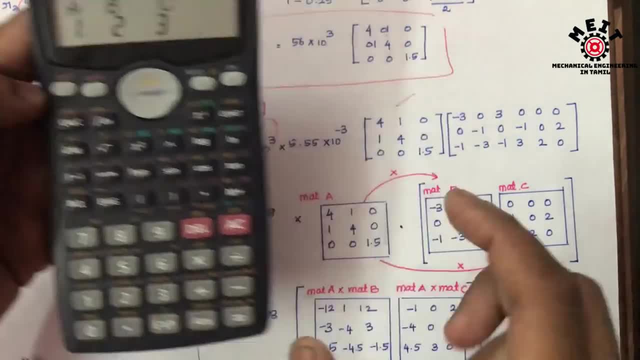 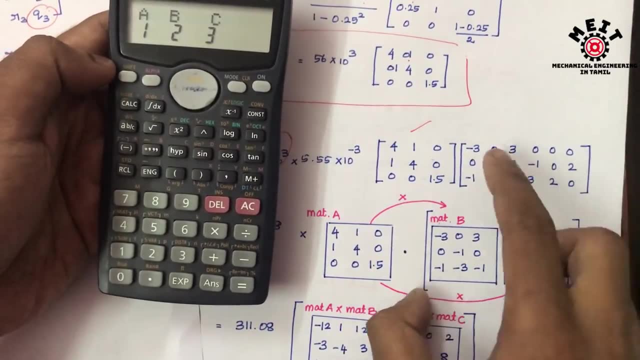 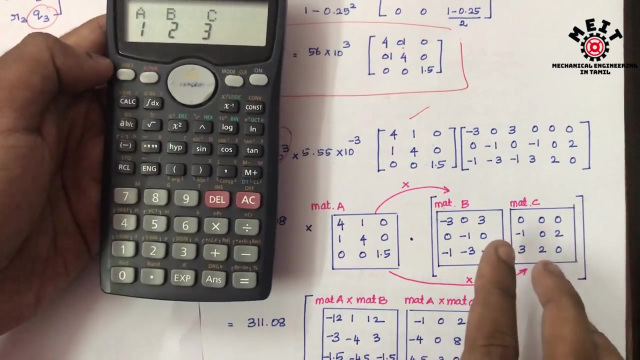 which matrix first, dimension number 1, we can save 3: matrix A, B, C. what I will do like I will take matrix A, then 6 cross 3, what I will take: matrix B, matrix C I have divided like box. no need to put box, just take as that. 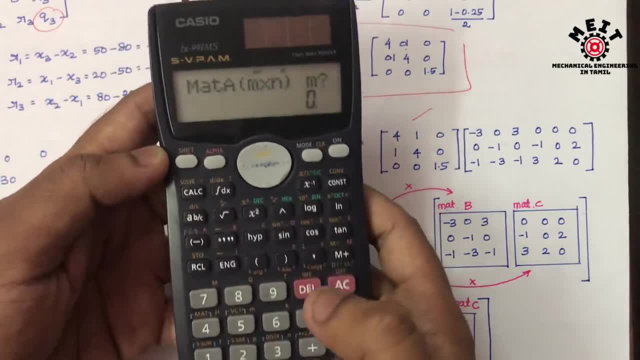 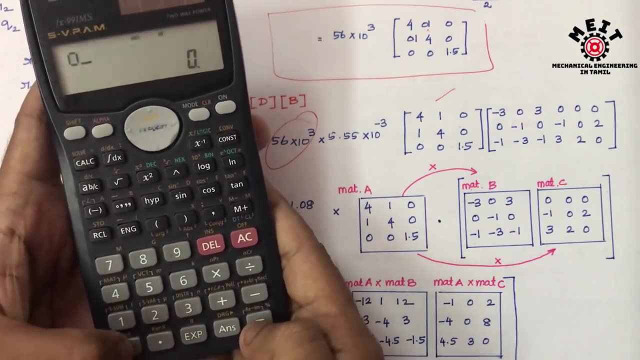 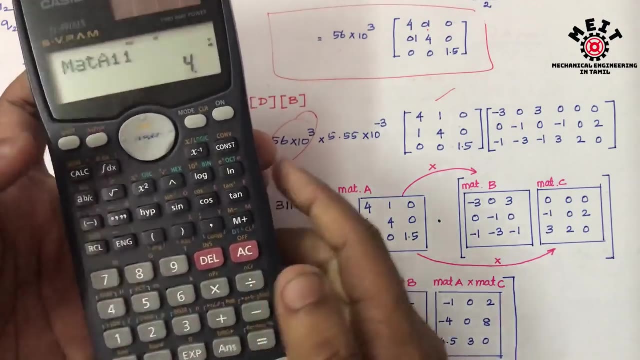 now, when I define matrix A, after giving 1 matrix A, 3 cross, 3 matrix 3, then 3 matrix value 4, 1, 0, 1, 4, 0, 0, 0, 1.5. now I define matrix 1. 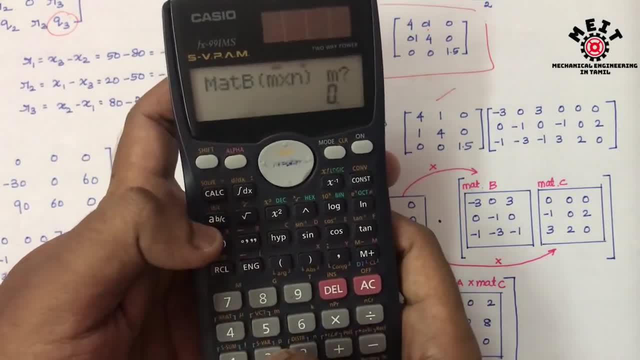 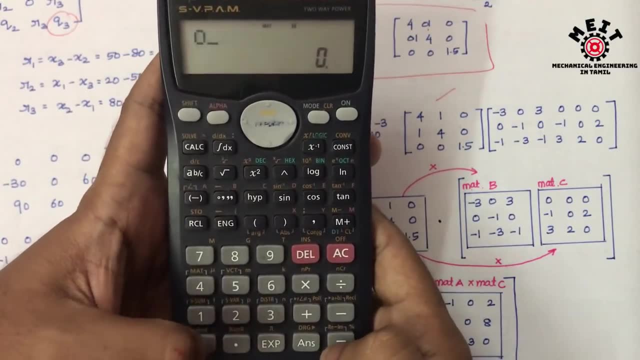 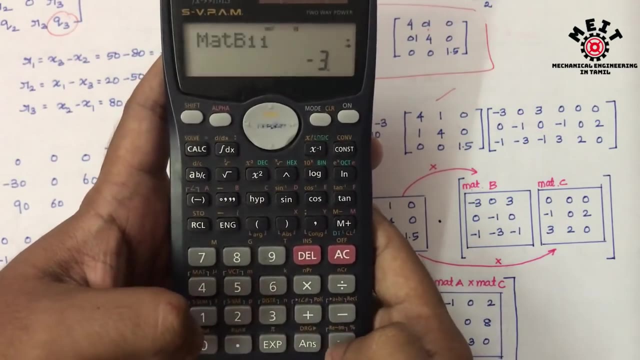 similarly again shift 4 dimension. matrix B 3 cross 3 minus 3, 0, 3 0, 3 0 minus 1, 0 minus 1 minus 3 minus 1, so matrix B 1 is saved. similarly, shift dimension 1. 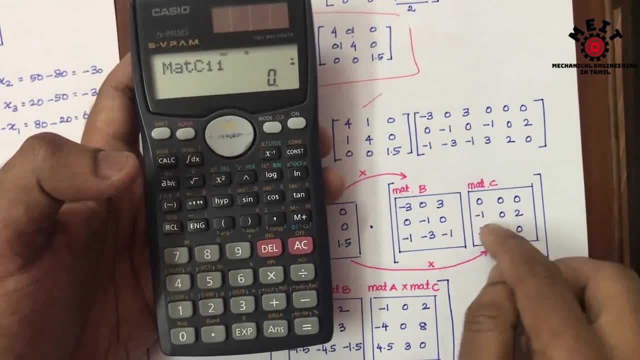 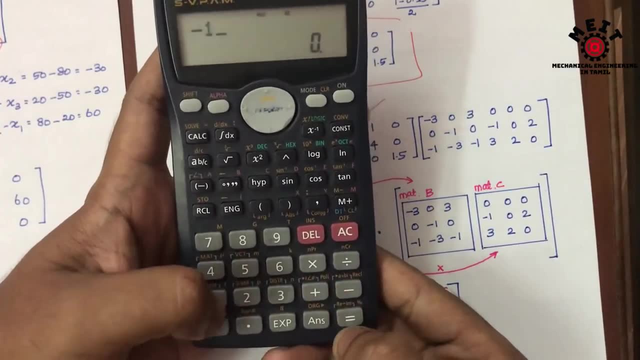 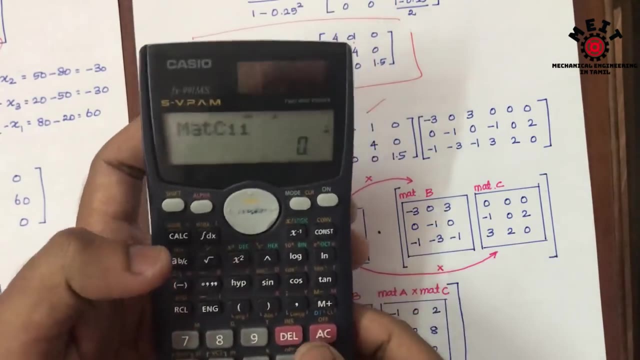 matrix C: 3, cross 3: how to save like 1, 2, 3, 1, 2, 3, 1, 2, 3, 2, 2, 3, 2, 0, 6, 6, 7, 8, 7 8. 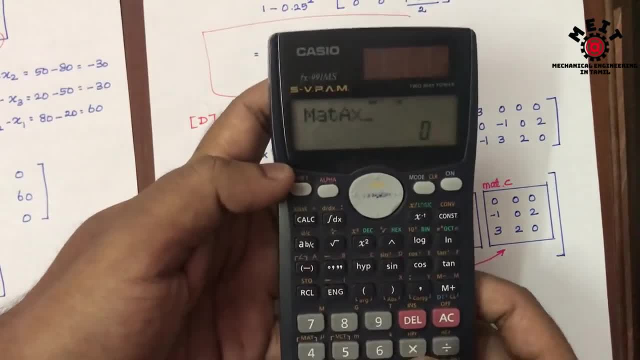 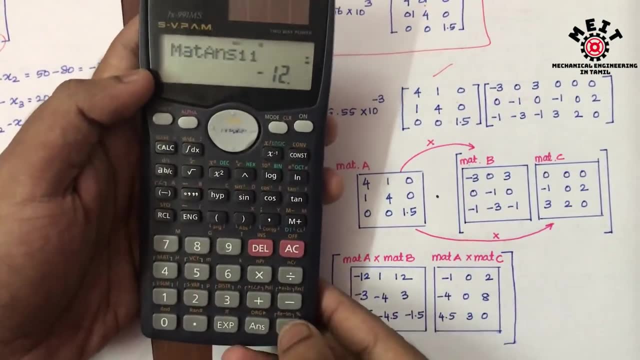 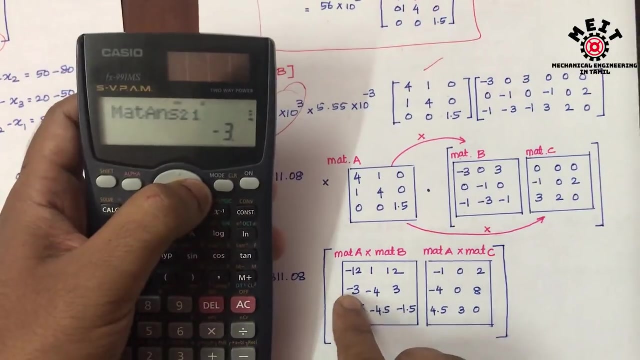 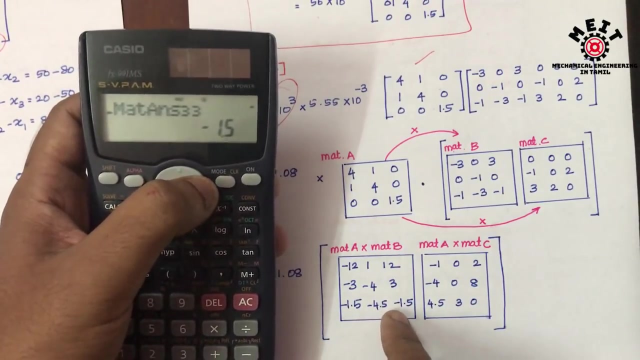 9, 10, 11, 12, 13, 14, 15, 16, 17, 18, 19, 20, 21, 22, 23, 24, 25, 26, 24, 4, 3, minus 1.5, minus 4.5, minus 1.5.. So if we divide the 3 matrices like this, if we multiply: 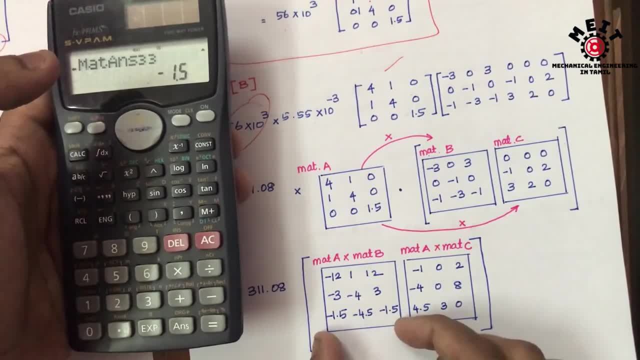 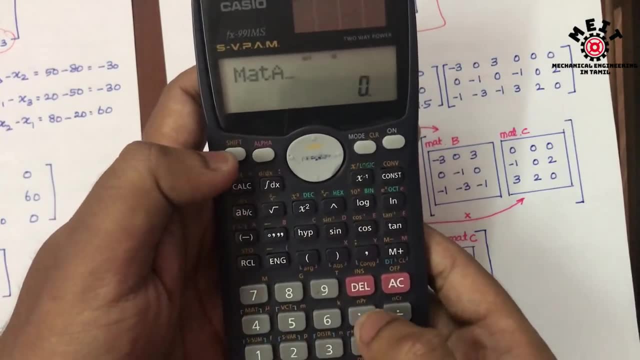 A and B. the answer will be here. So that will be the answer for a particular portion. If we want this portion, we have to multiply A and C. So similarly, I have taken 4,, 3, matrix A into shift. 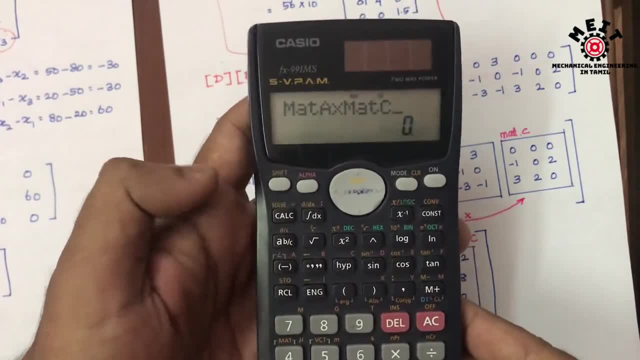 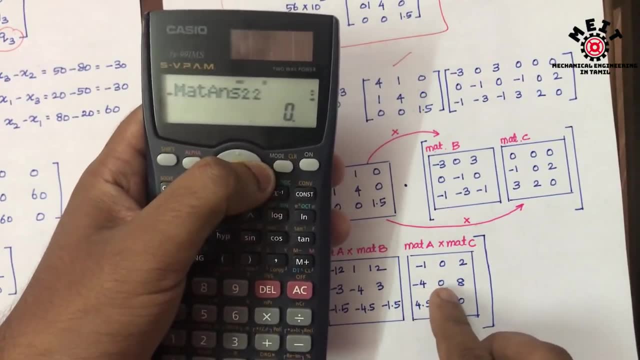 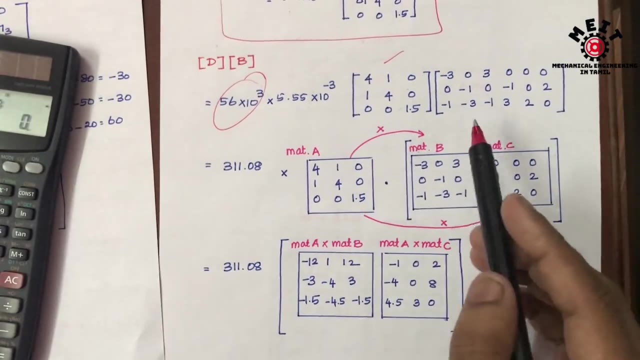 4, 3,. matrix C: If we multiply matrix A and C minus 1,, 0,, 2, minus 4, 0,, 8,, 4.5, 3, 0.. So this is the method to multiply: 3 cross 3 and 6 cross 3.. So if we multiply and finish, I can get. 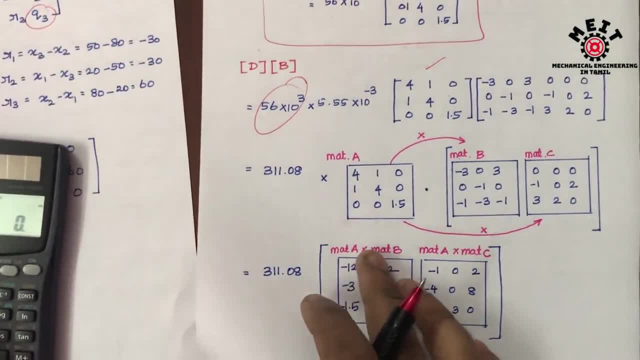 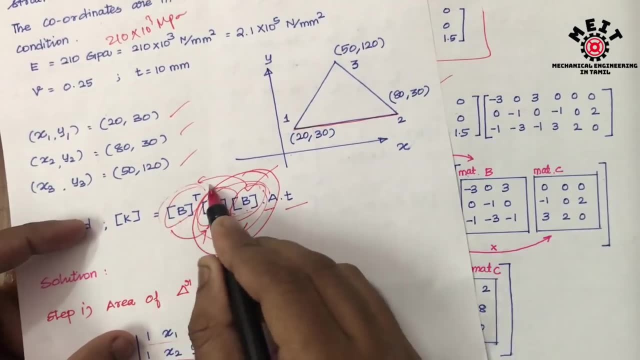 DB matrix. If we know DB matrix, what we will do next is we will find stiffness matrix Like stiffness matrix formula Bt, DB. We have finished calculating DB. Then we have to multiply Bt. So this is your Bt, Bt into: 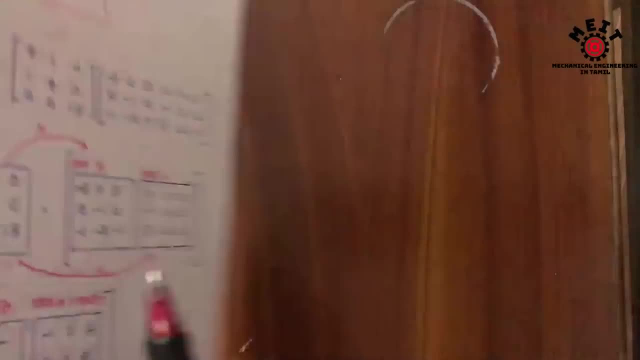 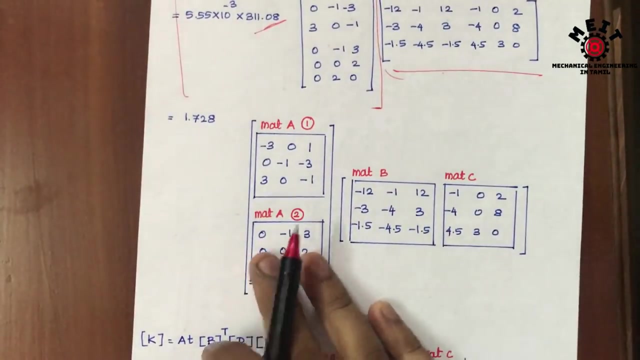 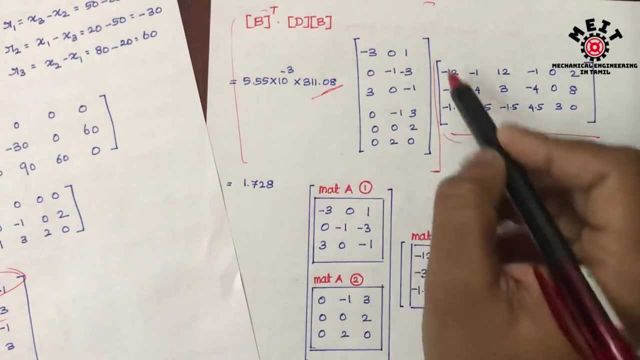 DB. What we do in DB is 311.08 into the matrix. So 311.08 into the matrix. So Bt is like 5.55 into 10 power minus 3 into the particular matrix. So 5.55 into 10, power 3 into particular matrix. 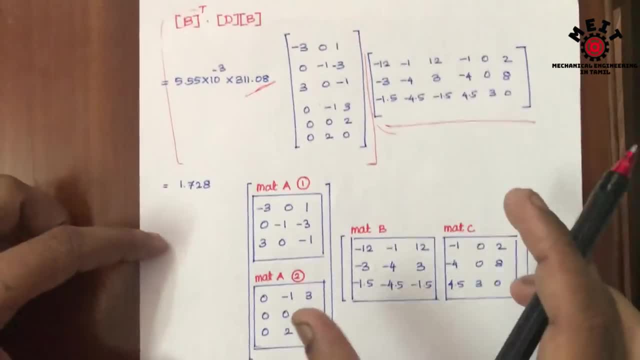 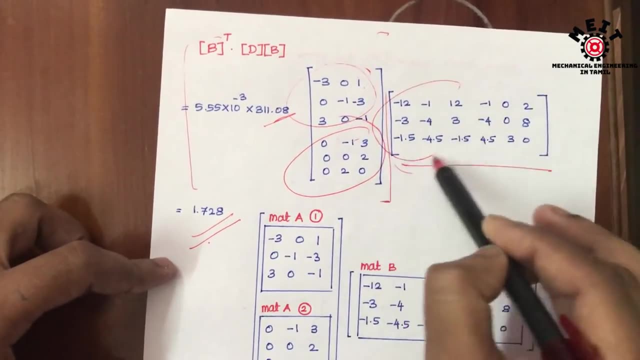 So how do we use this in CALCEL? I have to make the portion like this: I have to simplify it to 1.728.. Then I have to divide this portion into 4 matrixes. I have to divide this into 4 matrixes one by one. This is matrix A for. 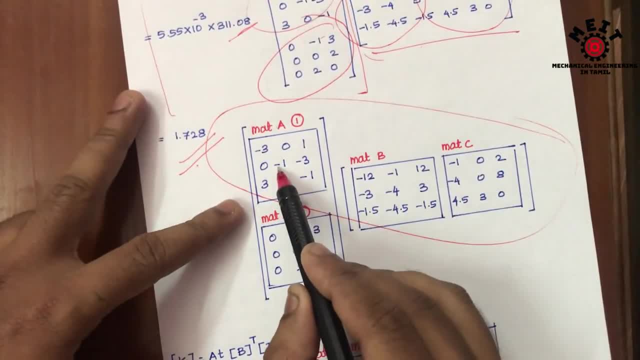 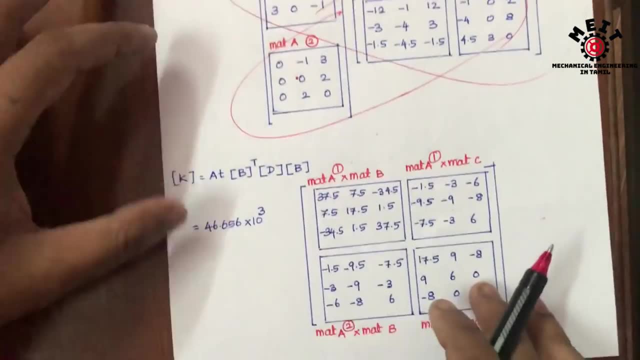 first calculation. First we have to do 2 calculations. First we have to take 1 as 1.. First A to 1.. Then A to 2.. Similarly, for the second calculation, we have to take 2 as A and B. So the final. 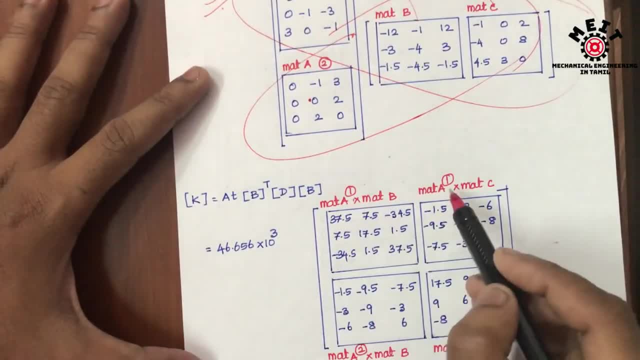 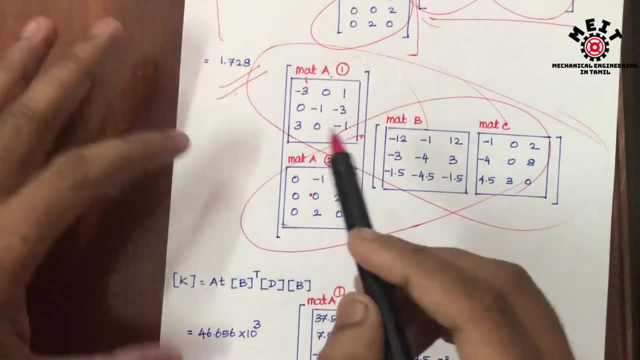 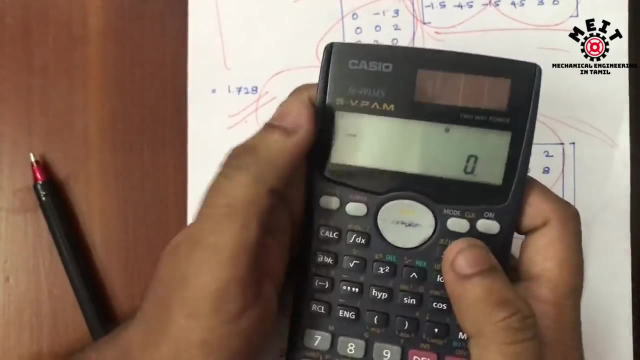 answer is: this is matrix A1.. This is matrix A1 into B and matrix A1 into C. This is the portion. So A2 matrix into B, matrix A2 into C. So first I will take A1 only, So after that. 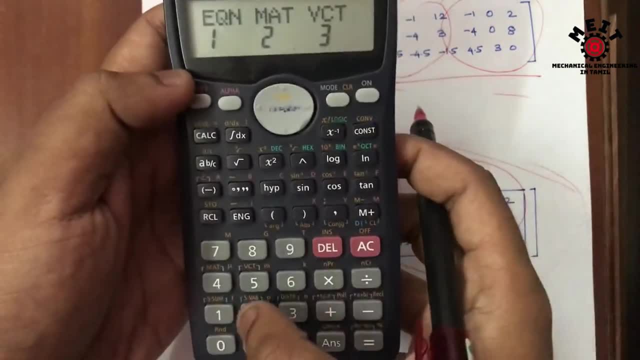 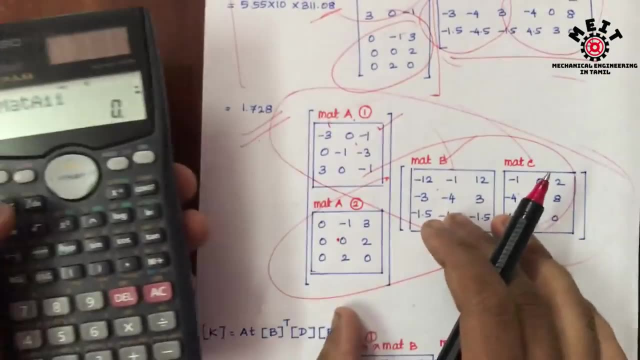 I will clear CALCEL. So now I am saving the matrix A Shift mode, matrix mode shift 4.. Then dimension matrix A, dimension 3, cross 3 matrix, So where it will be like minus 3,, 0,, minus 1, where is? 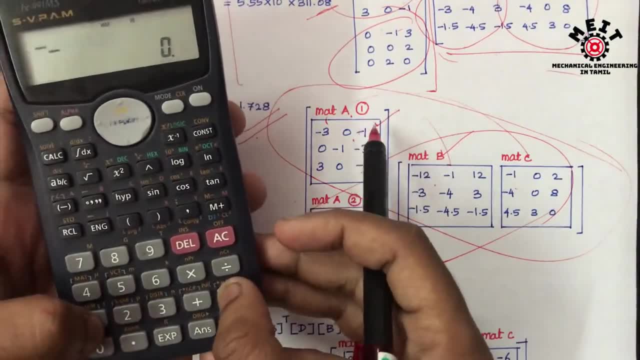 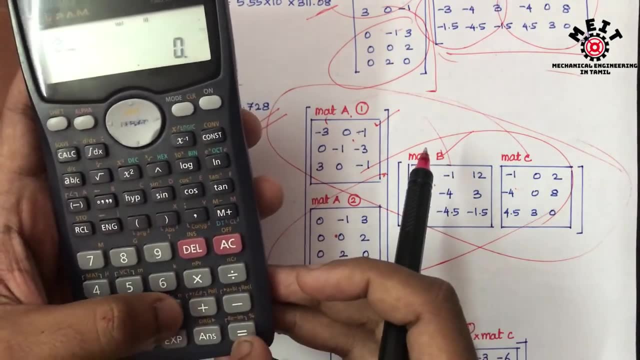 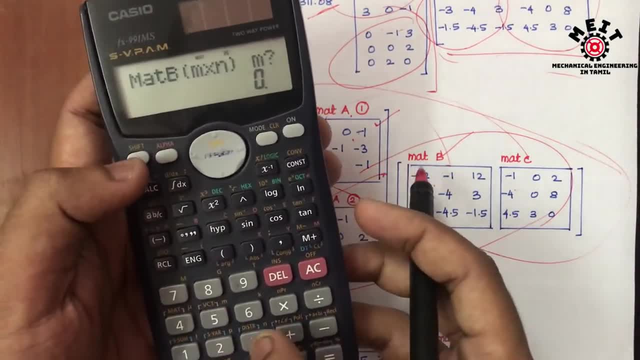 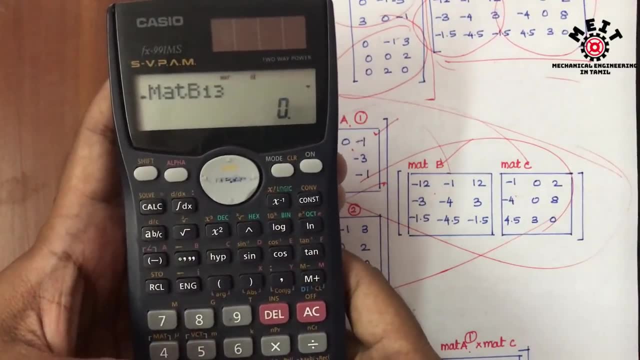 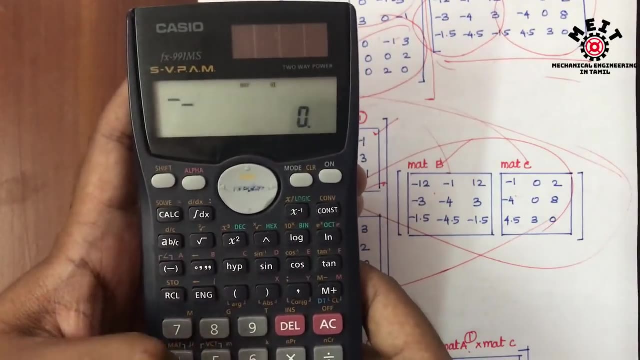 B, shift 4,. dimension: matrix B: 3, 3, class 3 matrix then: minus 12, minus 1, 12, minus 3, minus 4, 3, minus 1.5, minus 4.5, minus 1.5,. so matrix B is saved, matrix D is shift. 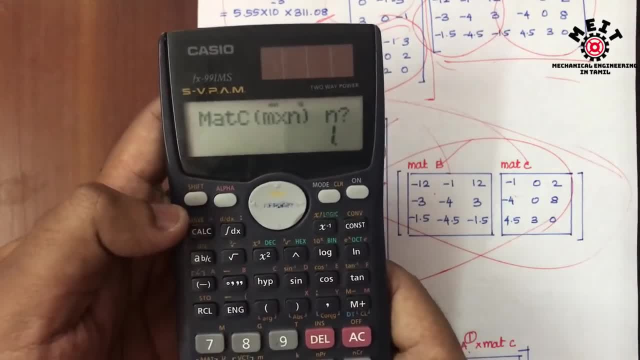 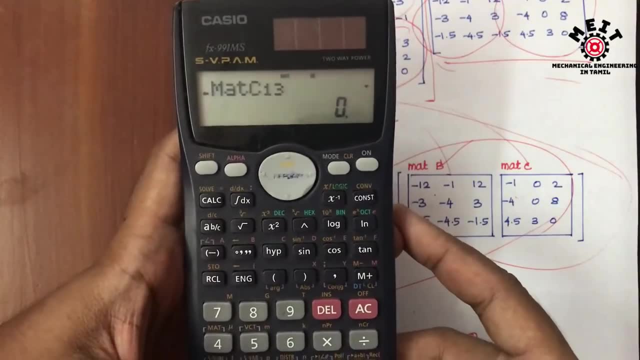 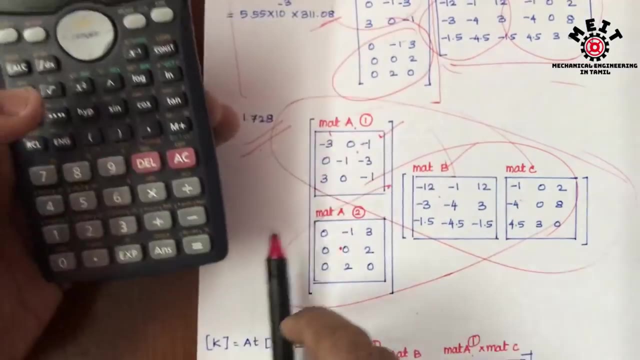 4, dimension. matrix C 3, class 3 matrix minus 1,. the matrix C is saved, minus 1, 0, 2, minus 4, 0, 8, 4.5, 3, 0, so I have saved 3 matrices. after saving, I am going to save the matrix. 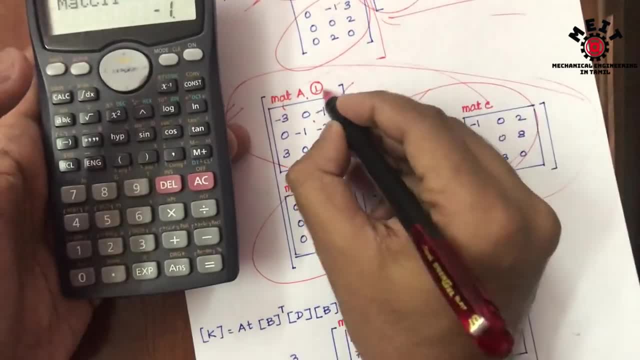 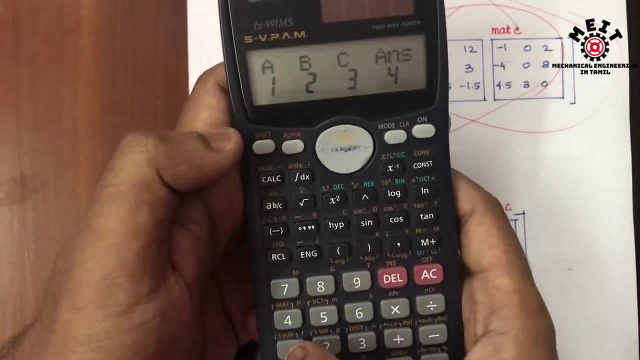 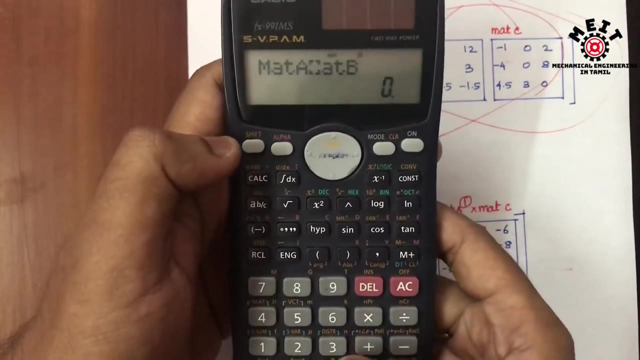 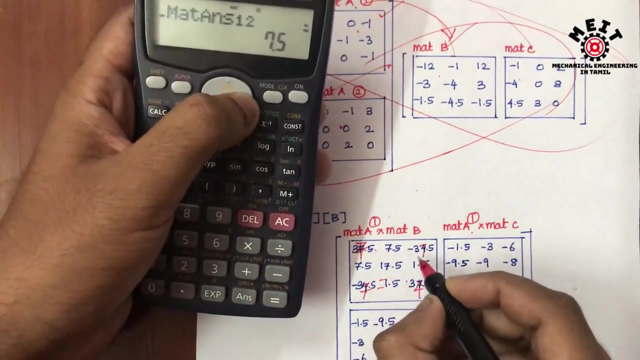 B, shift 4,. dimension matrix C: 3, 3, class 3 matrix minus 1, 12, minus 1, 12, minus 4, so I have saved 3 matrices. after saving, I am going to save the matrix B, shift 4,. 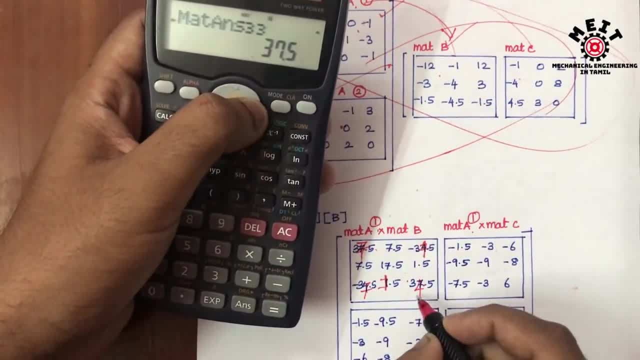 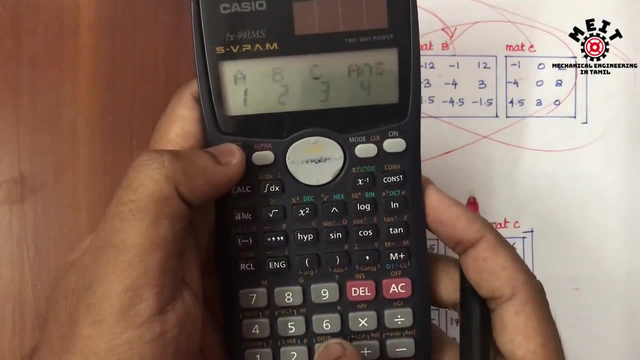 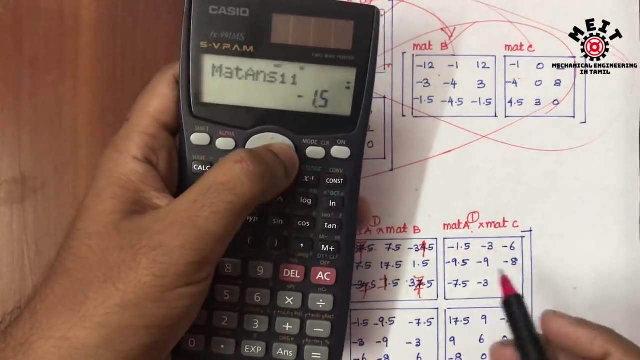 then minus 34.5,, then 1.5,, then 37.5, so that's it, and then shift 4, matrix A into shift 4, matrix C. if I do it again, minus 1.5,, minus 3,, minus 6,, minus 9.5,, minus 9,.